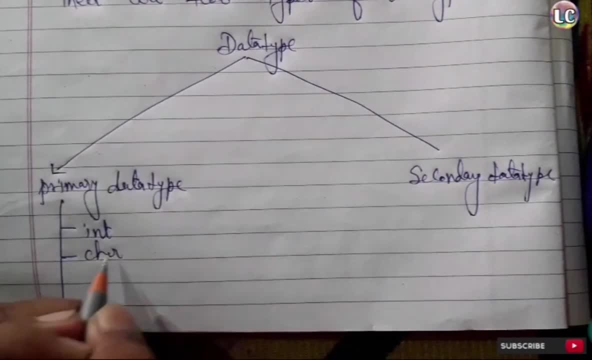 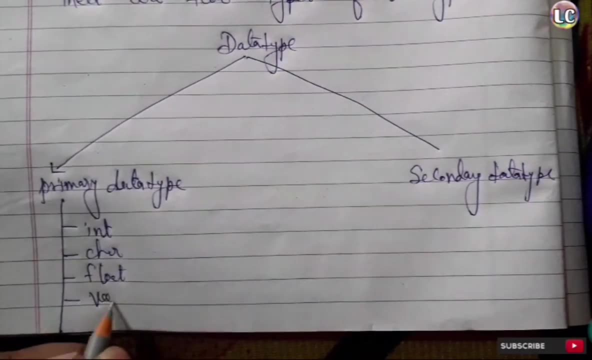 it is used to declare a variable. There is another definition which we can say that it is used to declare a variable. There is another definition which we can say that Care, which we use in our program, Int, care, float And last void. These are four data types. 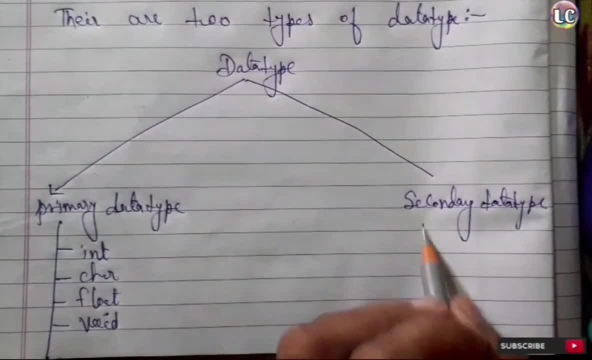 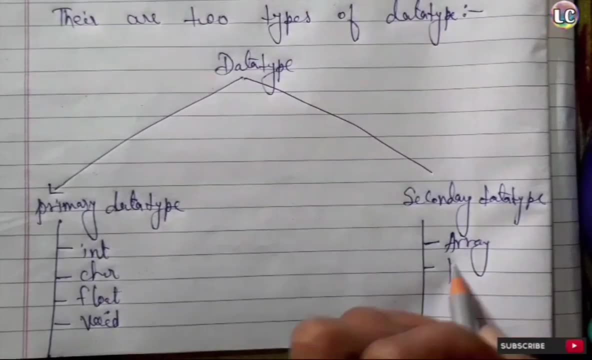 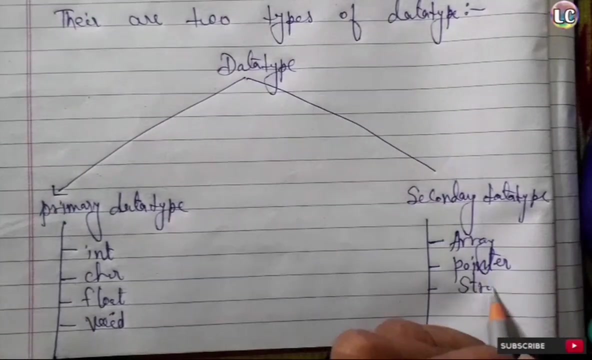 Which are primary data types. I will also tell you their size and range. Before that, let's see the secondary data types. First is array. After that we will write pointer. There are two more. Third is structure And fourth is union. Array, pointer, structure, union.